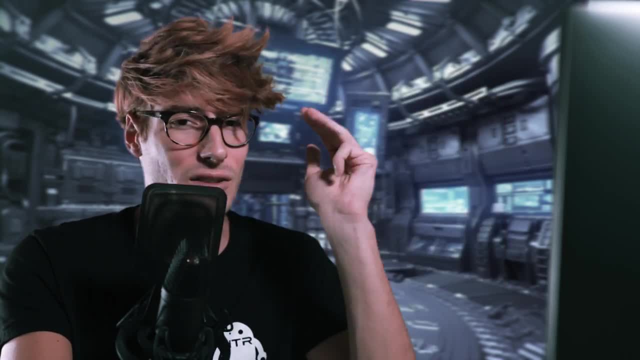 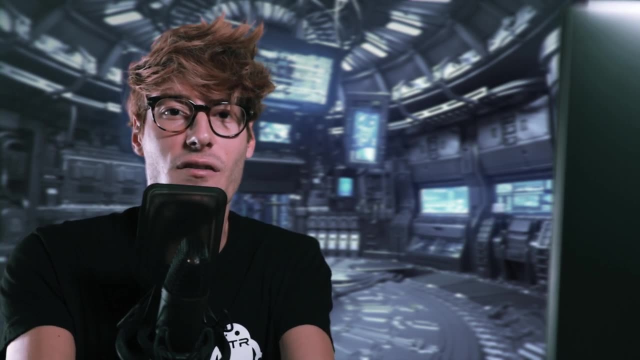 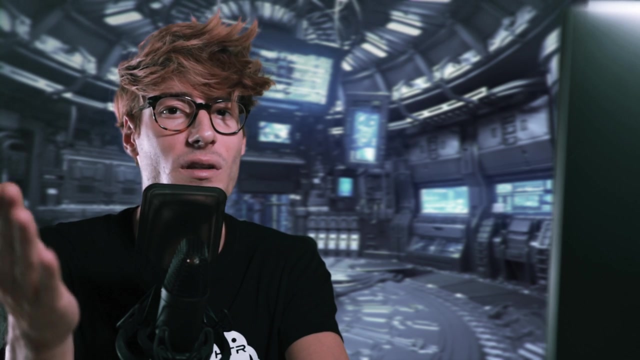 engineering, electronic engineering, information engineering, computer science, control theory, psychology and many others. So it's clearly impossible to specialize in every field, and it's better if you start focusing on few of them from the very beginning, while having just a general idea on what the others consist of. I'd say that we can group all the required competencies. 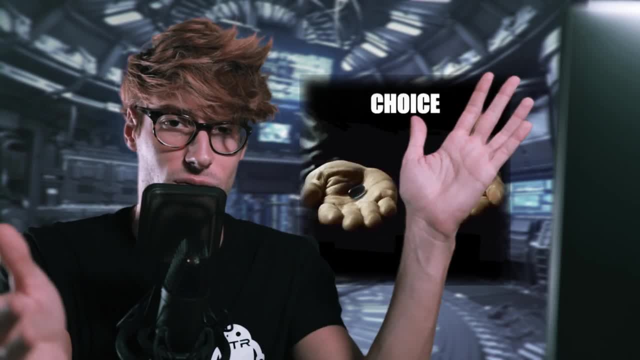 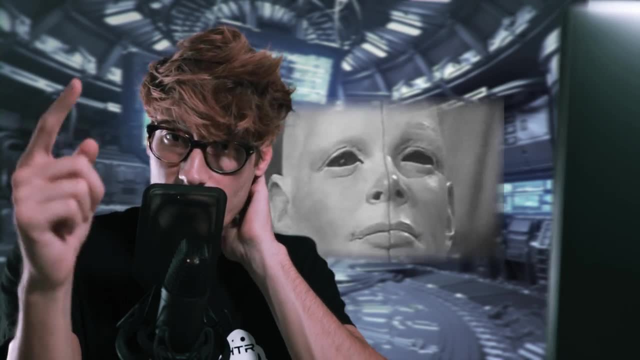 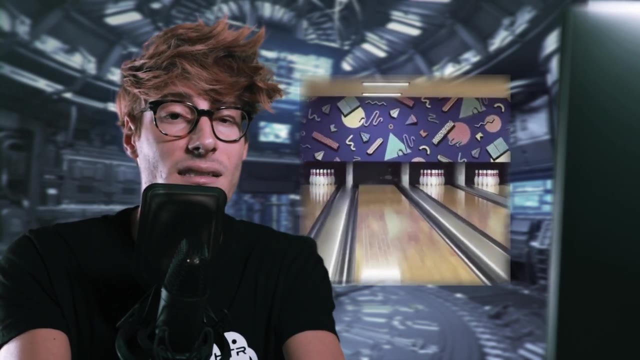 into main categories: Hardware and software. Hardware concerns everything about the design and realization of a robot. Electronics and mechanics are fundamental. Robots all have some kind of mechanical construction, formal shape designed to achieve a particular task, and they also have electrical components which power and 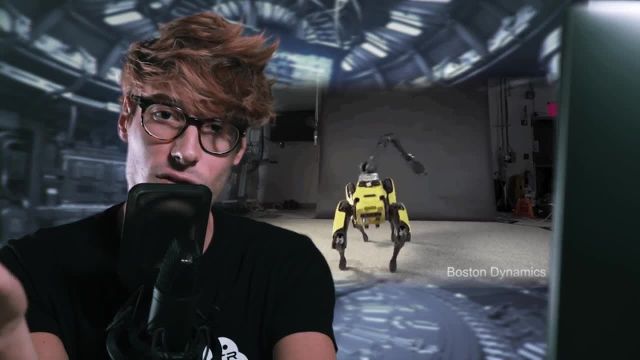 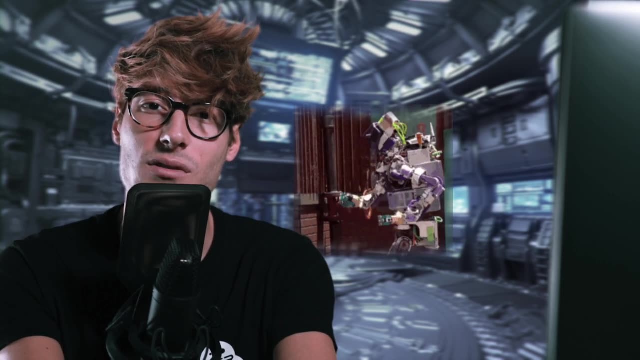 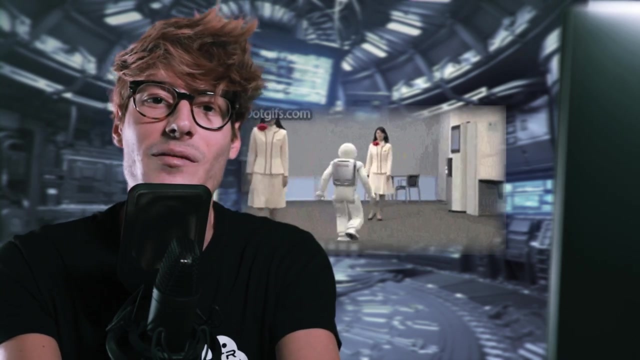 control the machinery. Software is about all the robot can do. All robots contain some level of computer programming code. A program is how a robot decides when or how to do something. Robots that use artificial intelligence, for example, interact with their environment on their own and can determine reactions to objects and problems they encounter. 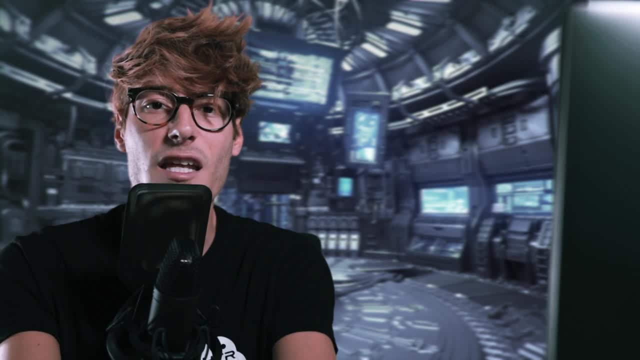 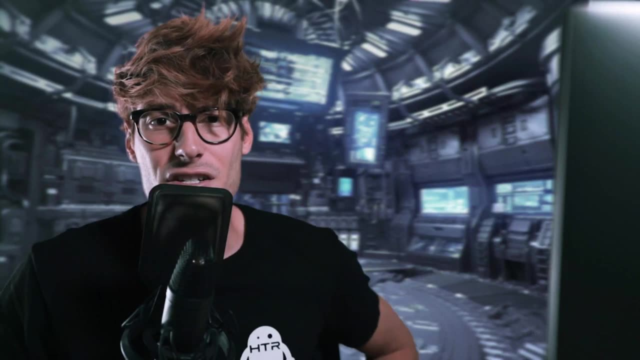 using their pre-existing programming. So it'd be wiser if you decide from the very beginning which one you want to go for: Software or hardware. If you're really interested in the hardware, I suggest you to first get a bachelor in electronics, mechanical engineering. 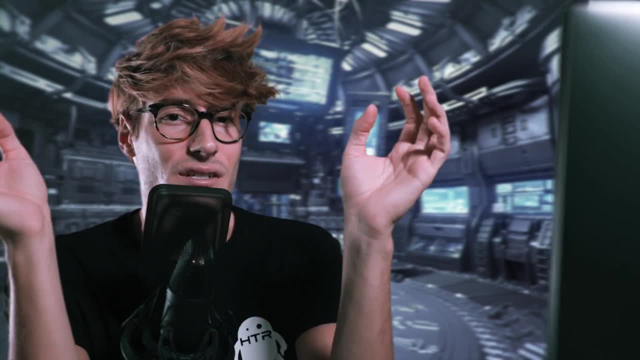 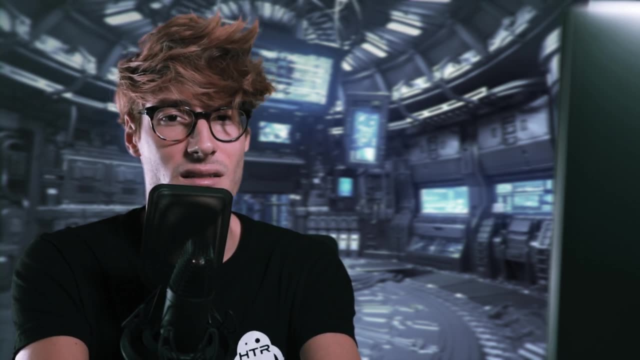 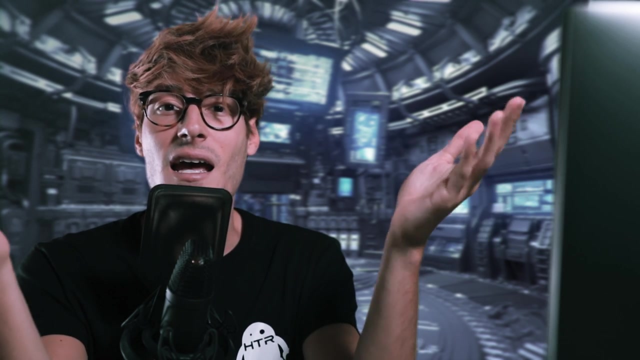 mechatronics or design engineering. The bachelor just gives a general overview on many subjects. so then you need a master of science to increase your knowledge in some specific areas. The master of science is really important, guys. In fact, the bachelor knowledge is not sufficient for you to become a good roboticist, and I don't even think it's. 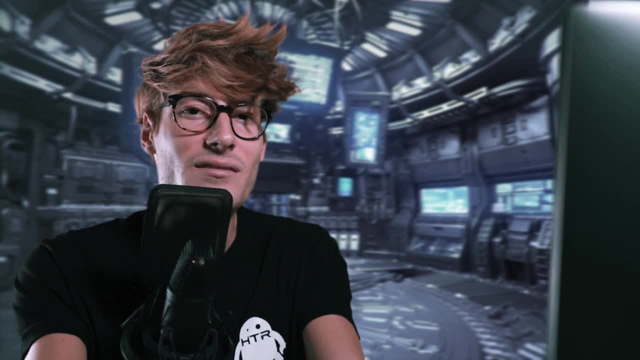 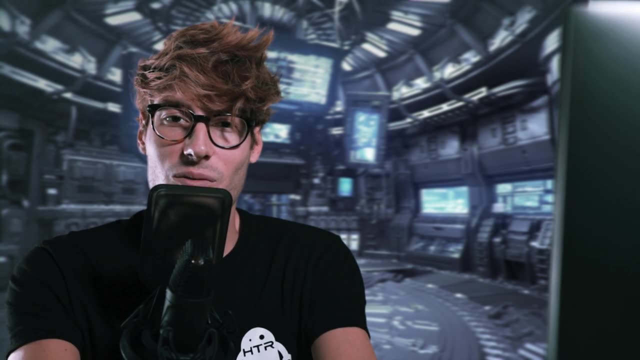 enough for you to get a job. Getting a bachelor is like reading the introduction of a book, so it's pretty useless. if you really want to understand the book, you know. So with a master of science, then you can get a robotics engineer job where you can provide technical support to. 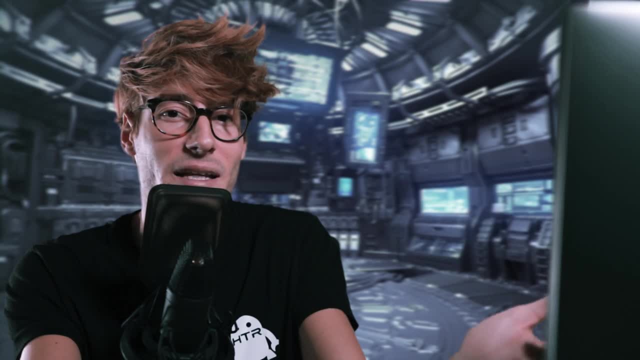 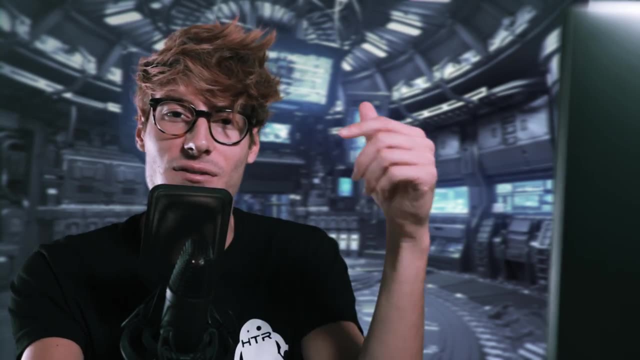 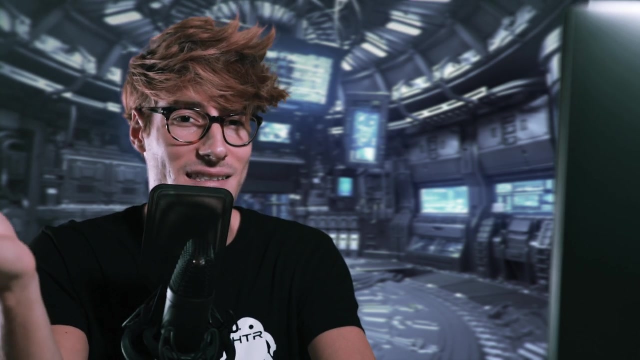 the robotics team, or you can start being a researcher in robotics, experimenting more innovative and completely new things. We can talk about the pros and cons of being an engineer versus researching in another video, I guess. So, to resume, the perfect path for someone interested in making robots would be to get one of the bachelors that I suggested, then a master of. 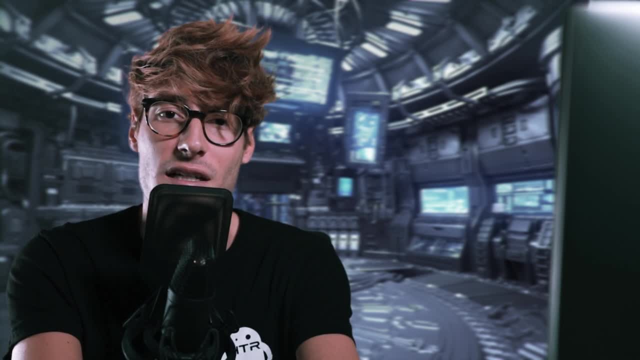 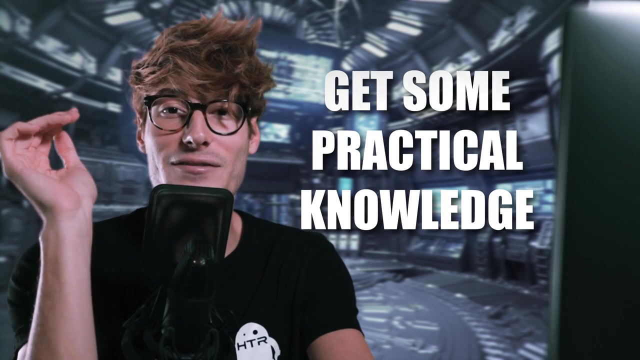 science that specializes in some particular areas of electronics, mechatronics or design. An example could be having a bachelor in electronics and then starting a master of science in embedded systems. So what's important, though, is that during your studies, you get some practical knowledge on robotics. Yeah, it's not said that you're gonna get it from the exams. 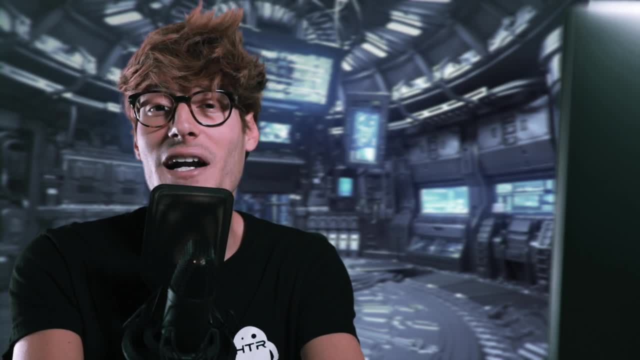 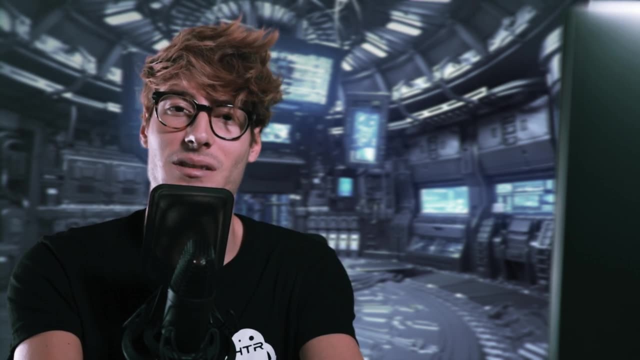 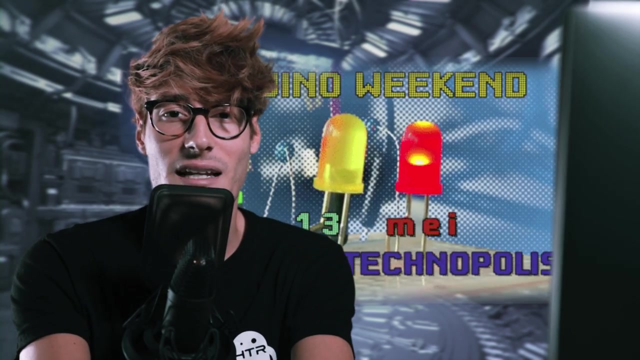 It's forced you to acquire some important technical background. that is very unlikely you get on your own, because it can get pretty lame, pretty actually really lame sometimes. So be sure you start building basic electronic circuits. you can start with things as simple as lighting up an led, then try more and more complex things by applying the theoretical concepts you 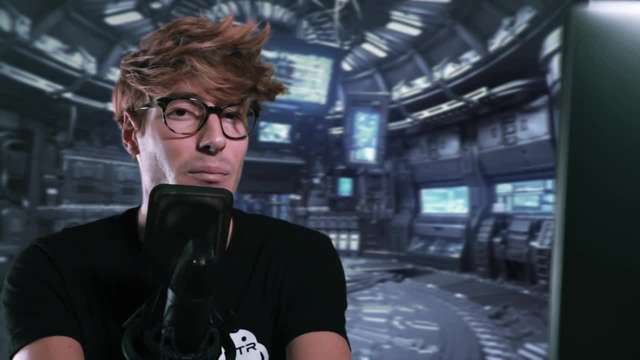 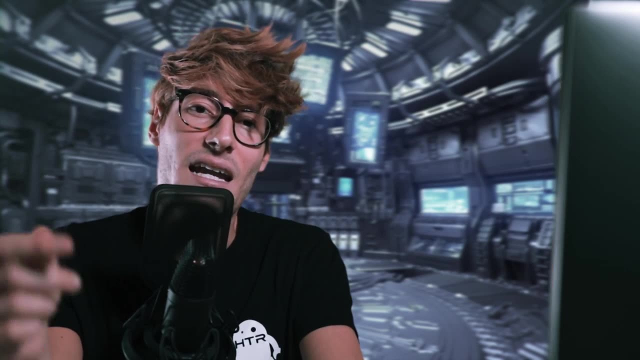 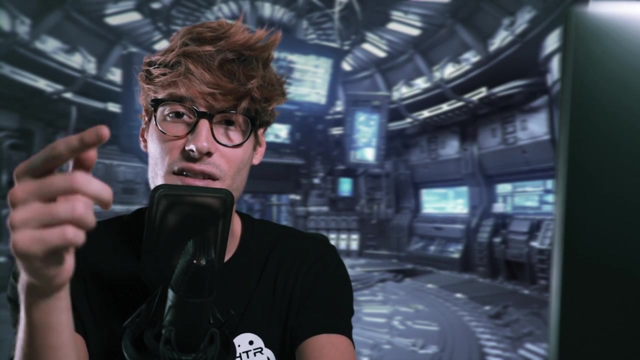 acquired during your studies. You can learn basic assembling, so learn to make some basic structures- wood, acrylic, fiber, plastic- and learn 3D printing. Start printing your own components, first by obligating some already existing projects online, and then experimenting new design on your 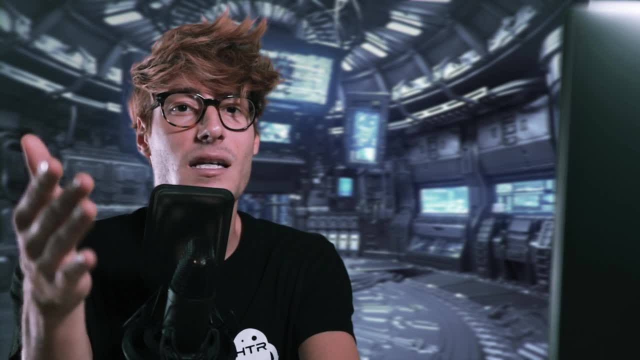 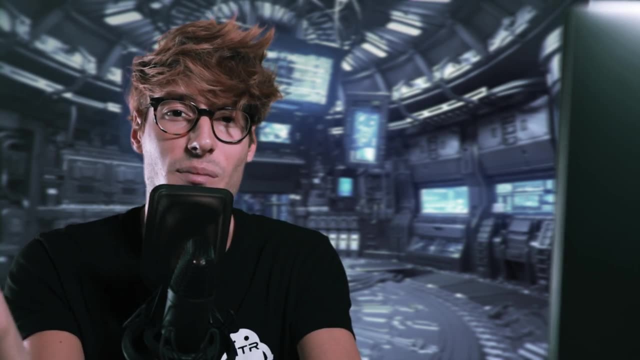 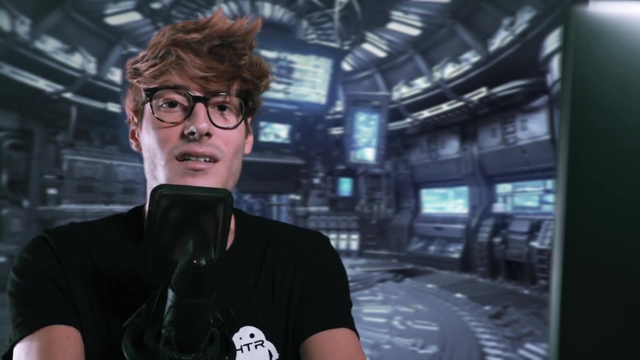 own. It would be cool if you can also integrate the above concepts with microcontrollers and try and test them on basic microcontrollers. The most popular choice among hobbyists and beginners is to go with Arduino. That's great and very simple. So learn CAD, you might be. 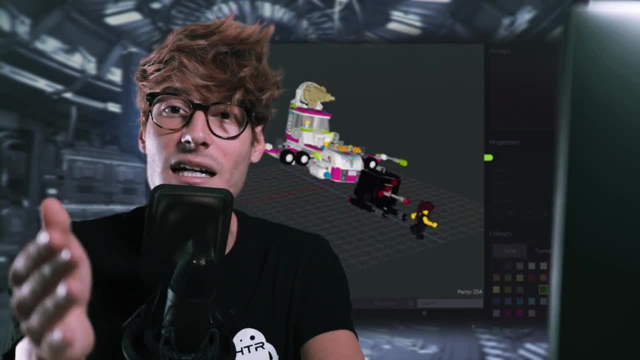 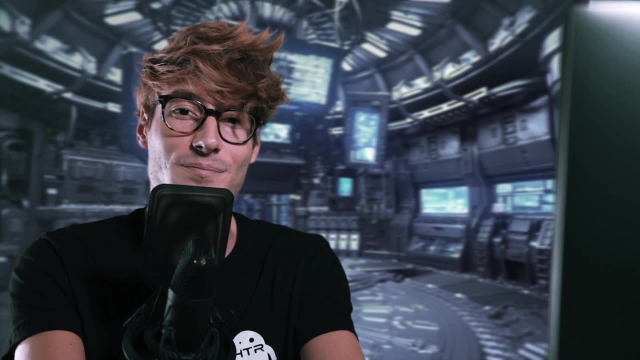 interested in learning how to use it. You can also learn how to use it on your own. You can learn to develop and design complex robots. so start learning 3D design software such as Blender or Solidworks, so that you can design your own robots. Well, these are only suggestions. you don't have to. 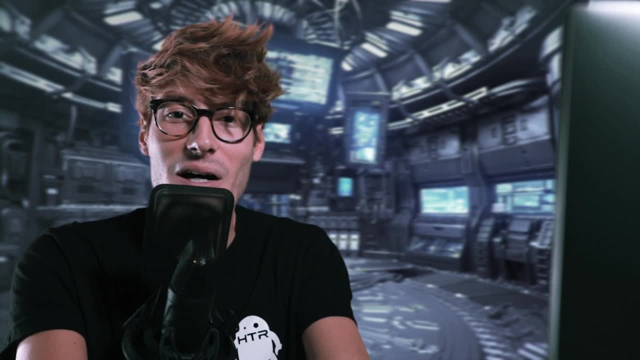 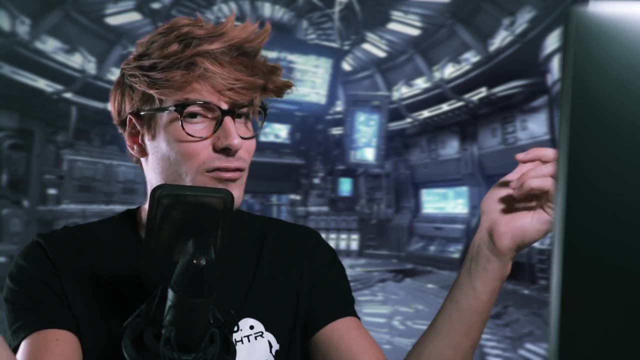 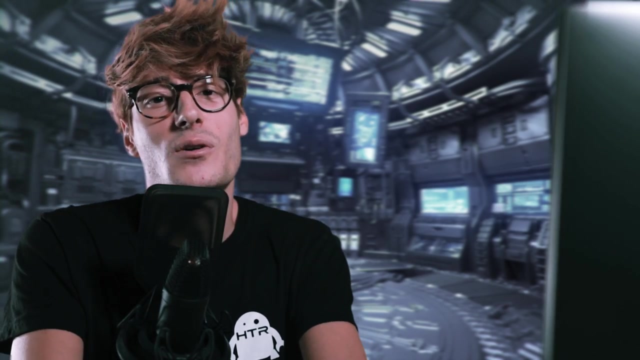 develop all these skills- I mean if you do better. but not all of them are strictly necessary. so I guess we can wrap up here with the hardware part. If you want to focus on the software part instead, you should first get a basher in computer science or automation engineering, and then you can get a master of science in artificial 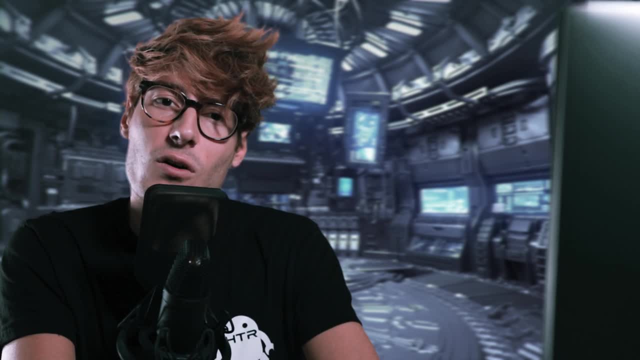 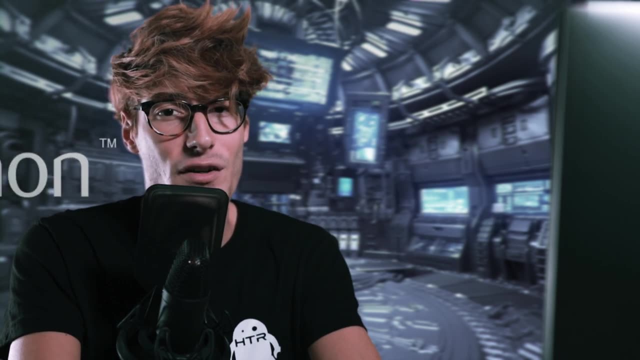 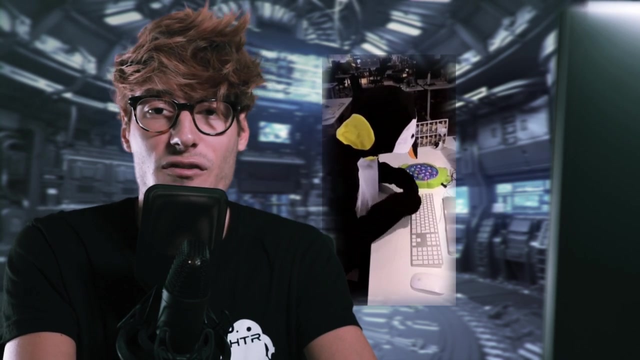 intelligence and robotics, or cognitive robotics, or automation and robotics. Among the competencies that you should develop, there are strong programming skills in C++ and or Python and confidence in using a Linux operating system. In fact, a lot of libraries, packages and software developed for robotics are distributed very easily and efficiently on Linux environments.